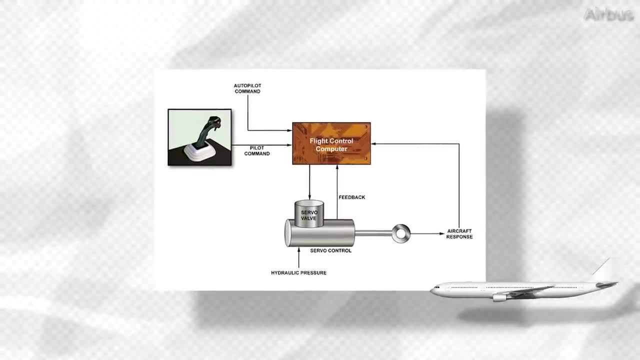 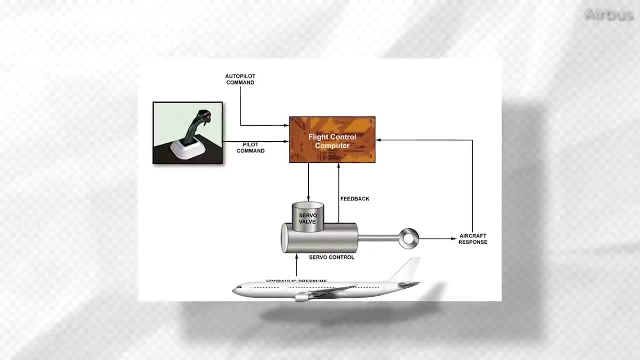 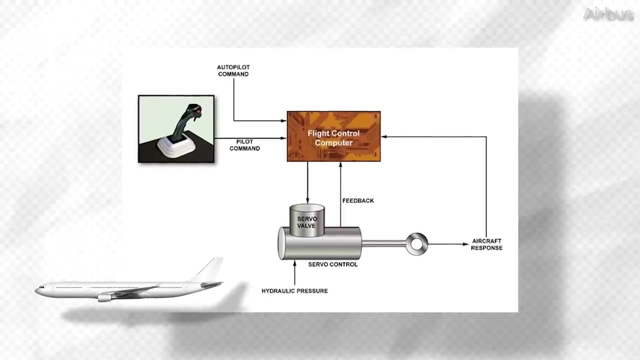 the FBW system translates the pilot's inputs into electrical signals. After processing the information received, these are transmitted to a computer that identifies the optimal way to activate the aircraft's control surfaces. No matter how hard Airbus pilots want their aircraft to pitch or roll, computer programming prevents the plane from performing maneuvers that. 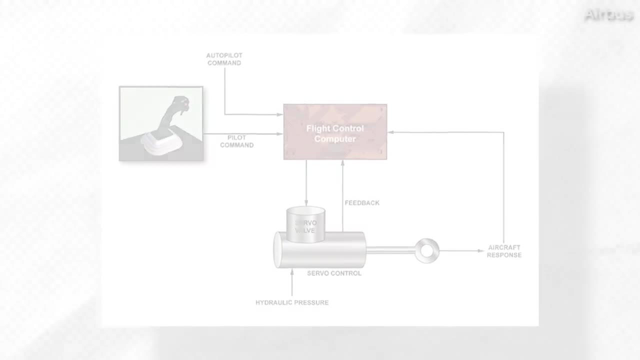 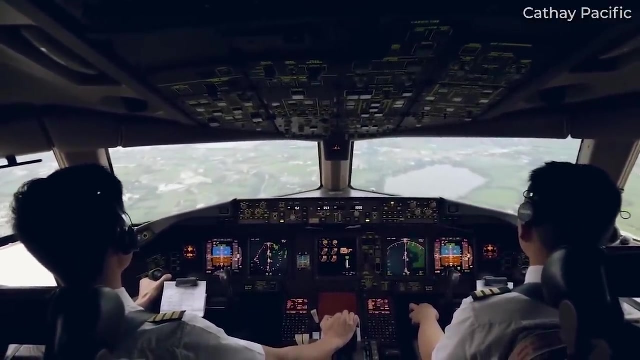 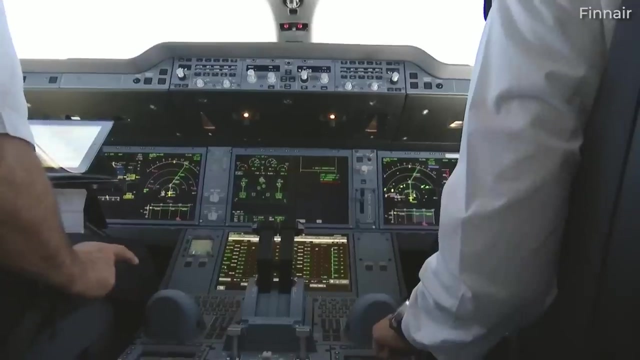 are considered unsafe at specific stages of the flight. In other words, assuming there were no aircraft issues where Boeing pilots could theoretically cause the aircraft to stall. their Airbus colleagues may find this more difficult, as an Airbus computer would prevent the aircraft from exceeding its operational. 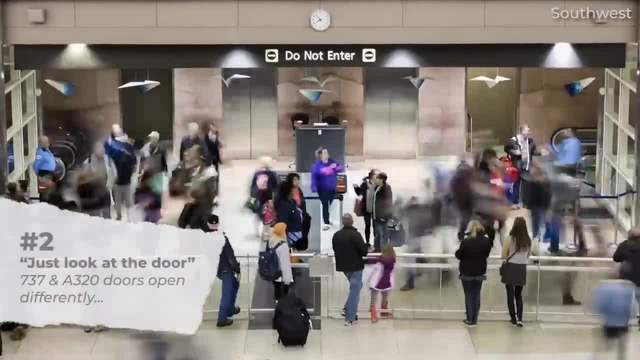 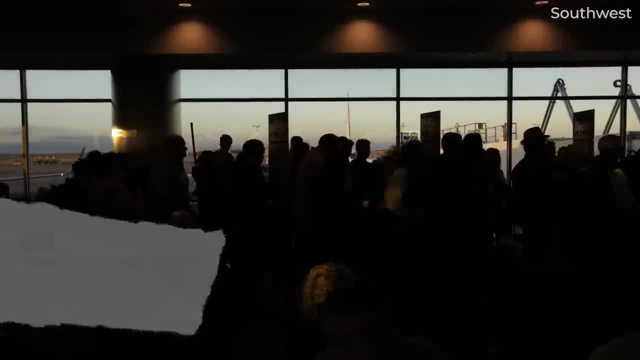 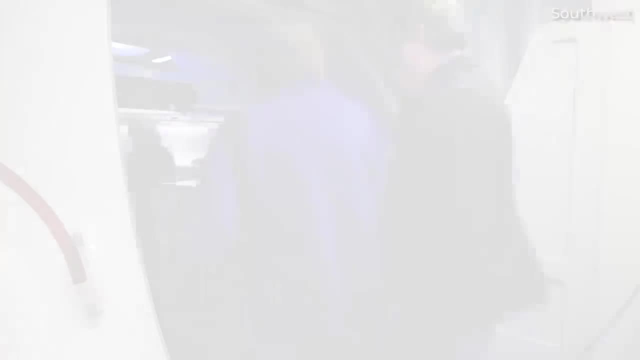 2. Just look at the door. If you're flying on a short or medium-haul aircraft and didn't have a chance to look out the window before stepping onto the jet bridge, it's still pretty easy to tell if you're on board an Airbus or Boeing plane as you approach the aircraft at the end of the tunnel. All you have. 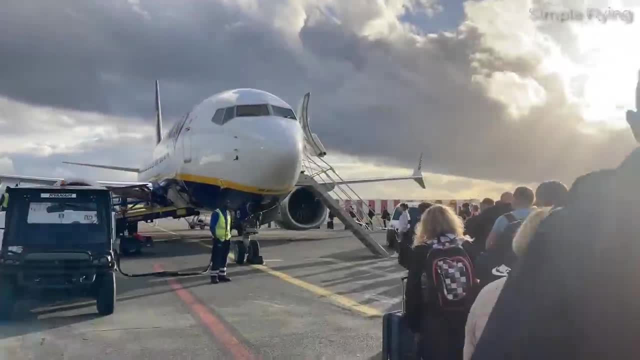 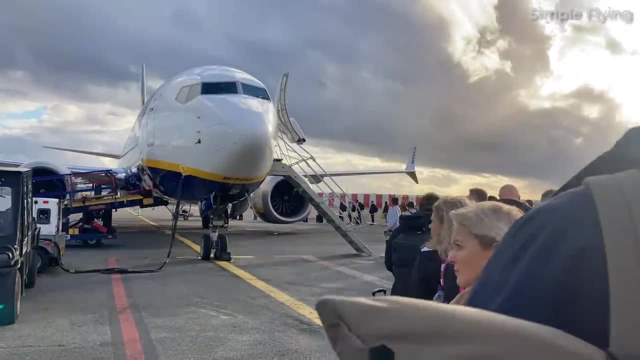 to do is look at the door while boarding. The Airbus A320 family and Boeing 737 family are the most popular short or mid-range aircraft. If you're flying on a short or medium-haul aircraft, you can get a close-up of the aircraft. If you're flying on a long or medium-term flight, 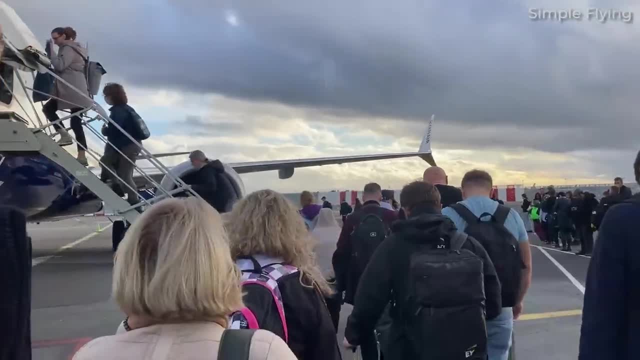 you can get a close-up of the aircraft by pointing at the door. If you're on a short-term flight, you can get a close-up of the aircraft by pointing at the door. However, they differ in many ways. One of the most noticeable is how the aircraft's doors are designed. Airbus doors run parallel to 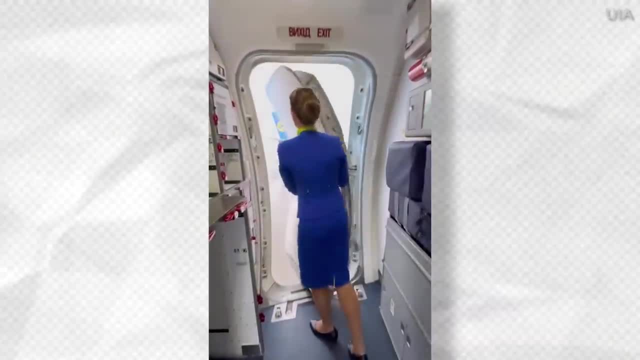 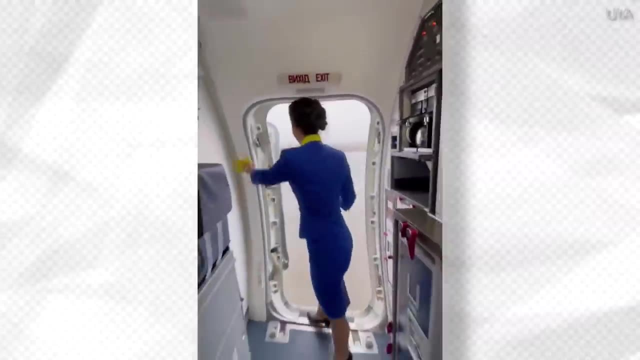 the fuselage when opened, while a Boeing door moves crossway, flipping open and exposing its cabin side. Additionally, opening a Boeing door almost always implies turning a lever, Whereas to open an Airbus door the movement is from the bottom up. 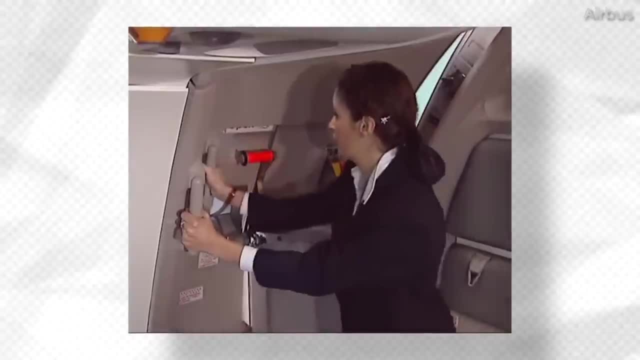 3. Turn the lever up and down. If you're flying on a short-haul aircraft, you need to look at the camera. You'll see that- the these different designs- it would appear that cabin crews need to put a lot more effort into. 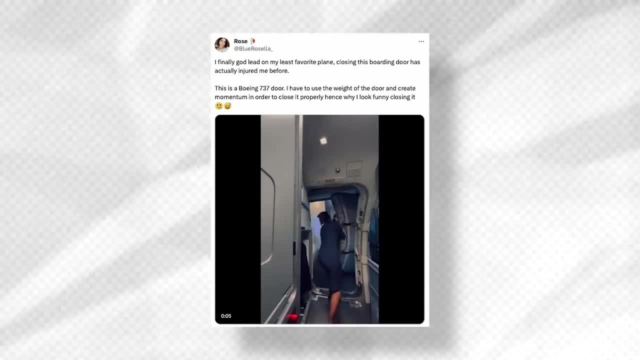 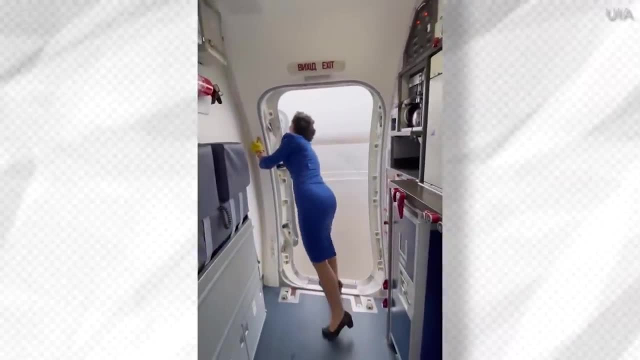 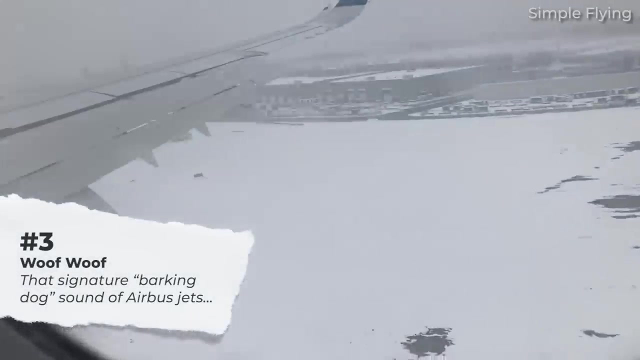 closing the door of a 737 than compared to an A320.. That's how it looks at least. If you've ever had the experience of closing a 737 door, do let us know in the comments down below what it's like 3.. Airbus' Signature – The Barking Dog Sound. 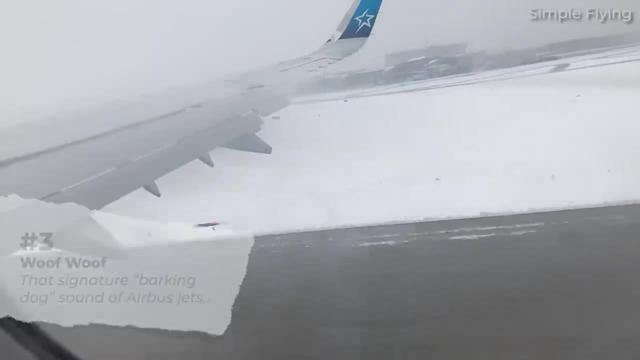 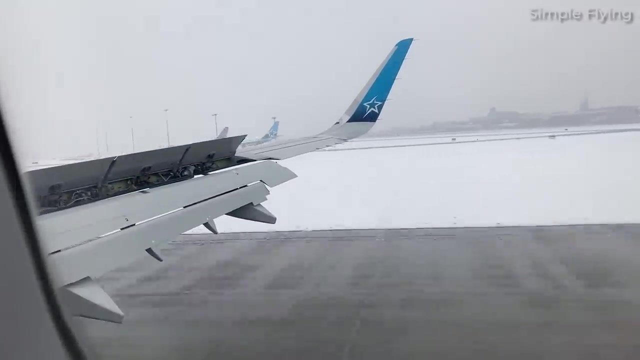 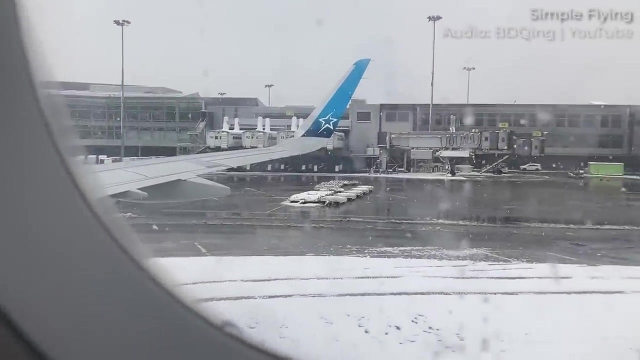 If you fly on an Airbus A320 family aircraft or an Airbus A330,, you will most likely hear what's described as a dog bark sound at specific stages of the flight. If this is the case, you have nothing to worry about. The sound is indeed a sign that the 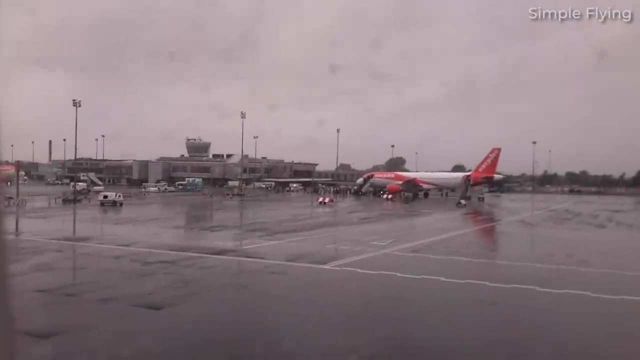 aircraft's hydraulics are functioning correctly. Phenomenal news, right As it happens, this unusual noise is causing the aircraft to bark. If you fly on an Airbus A320 family aircraft, you will most likely hear what's described as a dog bark sound. If this is the case, do let us know in the 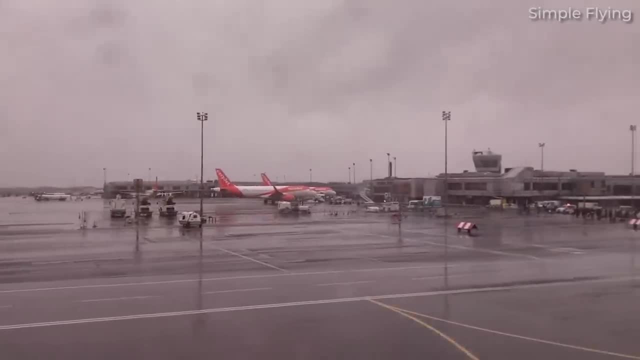 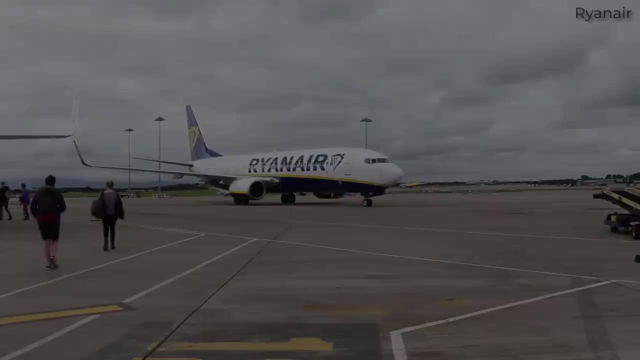 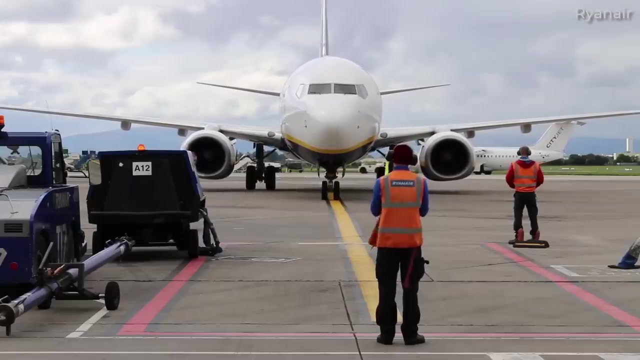 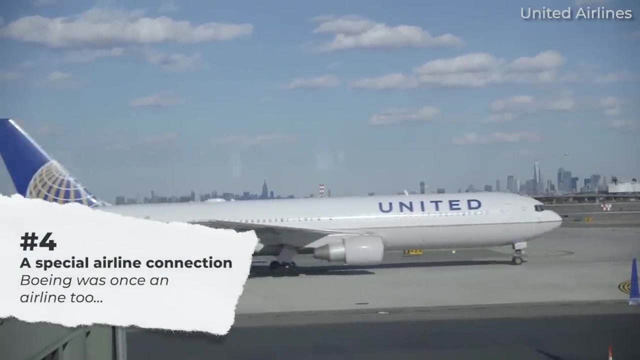 comments down below. If so, please hit the like button to help this video and share the information with your specialакаins and fans. Are we finished? Does this mean that, all així, two airbus carriers, one І-35 is no longer required? Perhaps? Here are some of the most important. 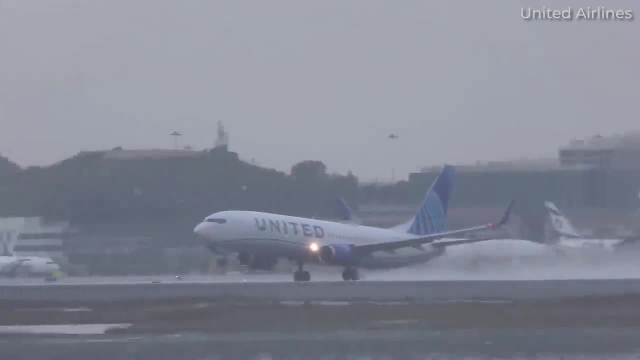 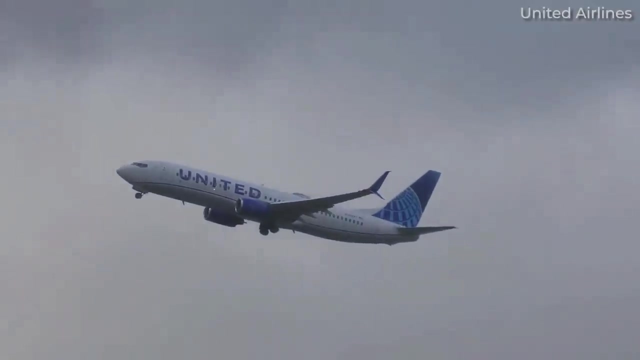 between their commercial aircraft products. let's look at some history. Boeing and Airbus have played a fundamental role in shaping commercial aviation as we know it today. Among the two expert manufacturers, however, there is one whose history dates back to the very early days of aviation. William E Boeing was an American timber. 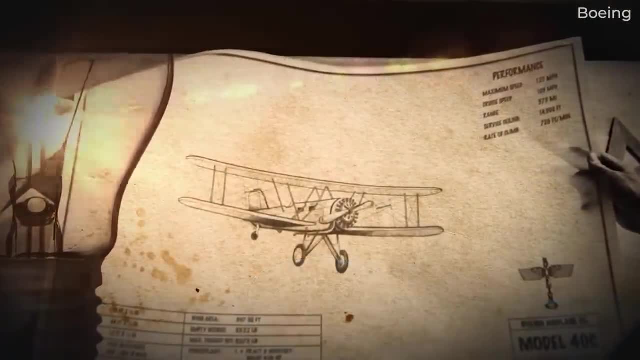 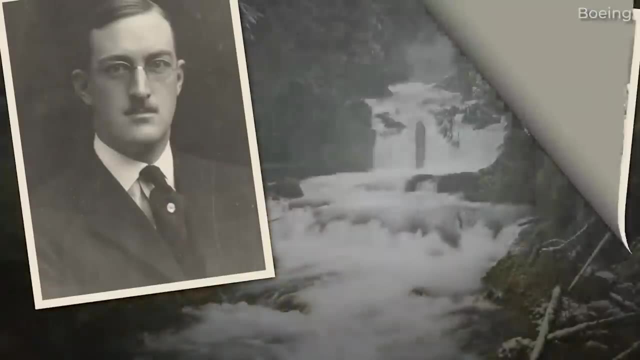 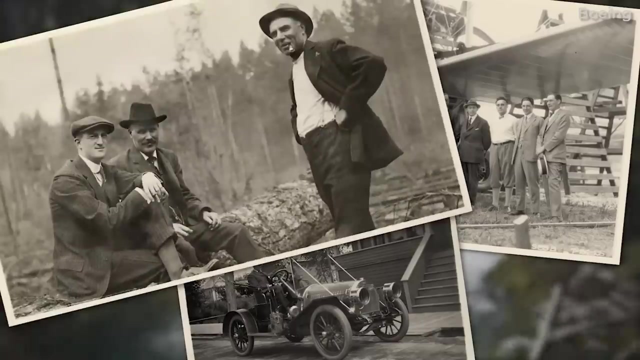 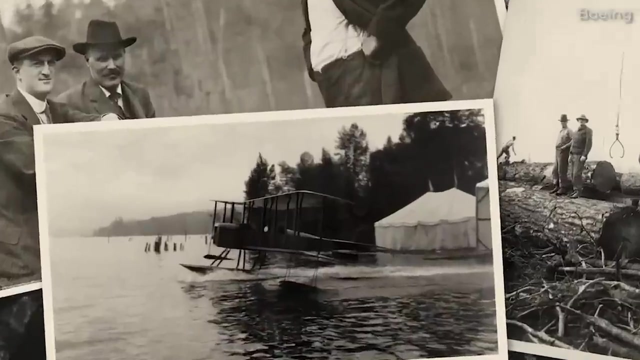 merchant who founded Aero Products Company after developing a single-engine, two-seat plane in 1916.. The following year the business name was changed to Boeing Airplane Company and it started manufacturing flying boats for the US Navy during World War I. After launching airmail services in 1928, William Boeing founded Boeing Airplane and 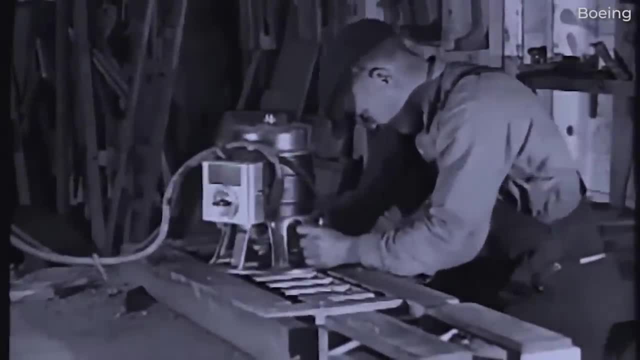 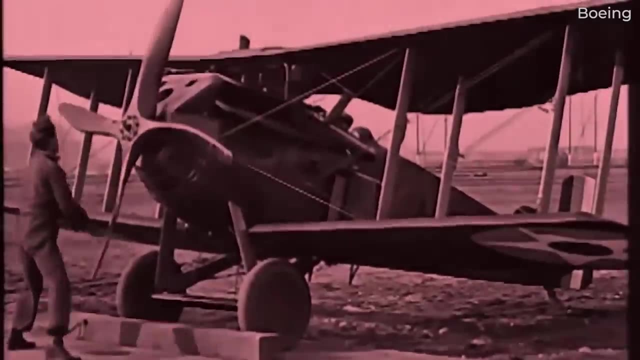 Transport Corporation to expand into airline operations. The following year, the company was renamed United Aircraft and Transport Corporation and acquired smaller aircraft makers and engine manufacturers. Boeing Squadron Th fame potentiallyOW 써idd is the Italianño femmìció del transport negozsieco, reporting a new industry three years ago. 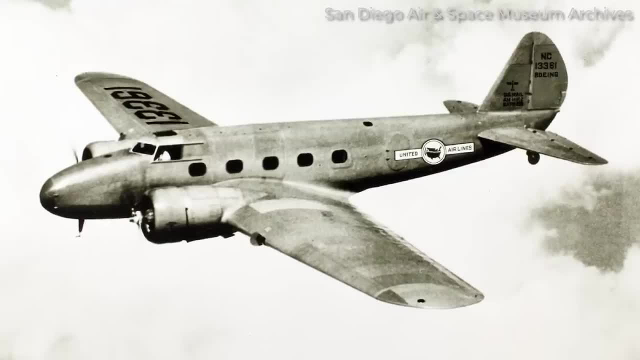 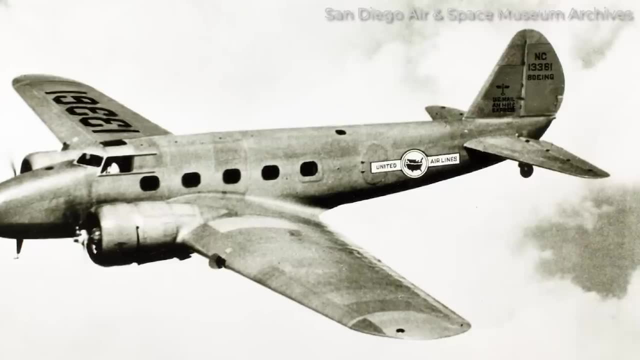 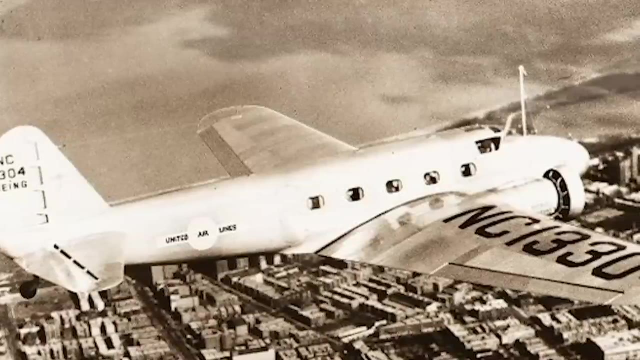 manufacturers, including Pratt & Whitney. In 1931, four small airlines were added to the business, giving birth to United Airlines. In 1934, the new US antitrust legislation prohibited aircraft manufacturers from being involved in air transport. Therefore, United